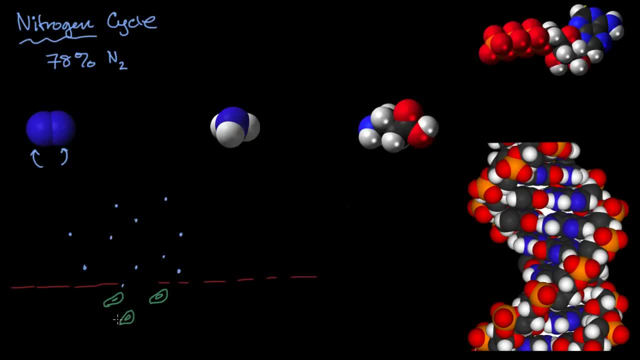 And certain types of bacteria are capable- and prokaryotes are capable- of fixing nitrogen. So what they're able to do is they're able to take that N2 and turn it into a form that is more usable by complex organisms like plants. 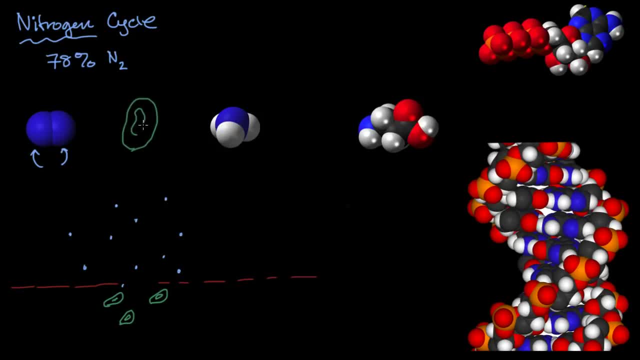 So this is the bacteria right over here. So that's the bacteria. That's just a little circular strand of DNA. I could draw other, I could make it more complicated, but let me just do it like this Bacteria is able to fix. 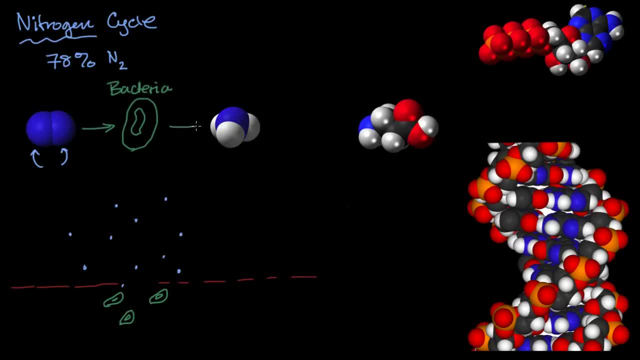 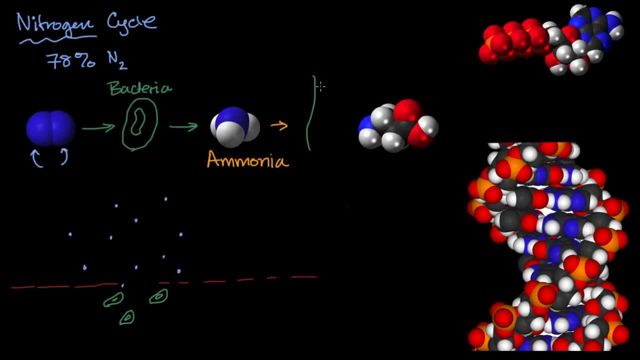 So this right over here. So as the plant in the video on the carbon cycle, we talk about how plants fix carbon. that carbon makes up a large part of organic molecules, But many important organic molecules also need nitrogen, And these are examples of organic molecules. 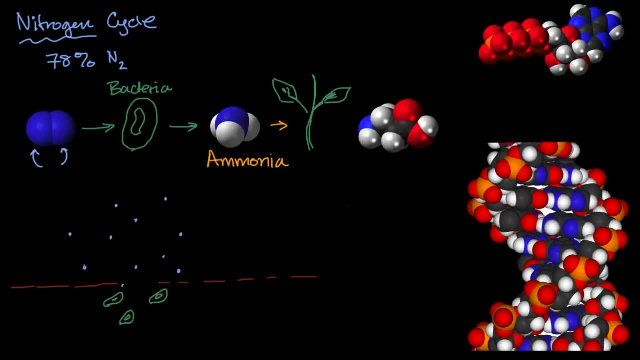 that you will find in plants, and you'll find them in many different types of organisms. So this right over here is an amino acid, Amino acid. You see the nitrogen right over there. This right over here is our good old friend ATP. 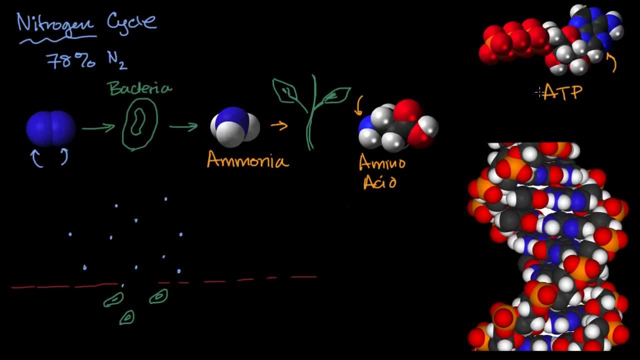 adenosine triphosphate. the store, the quick store of energy in biological systems. You see the nitrogen in blue right over here. You see the nitrogen in blue right over here. You see the nitrogen in blue right over here. This is the famous DNA deoxyribonucleic acid. 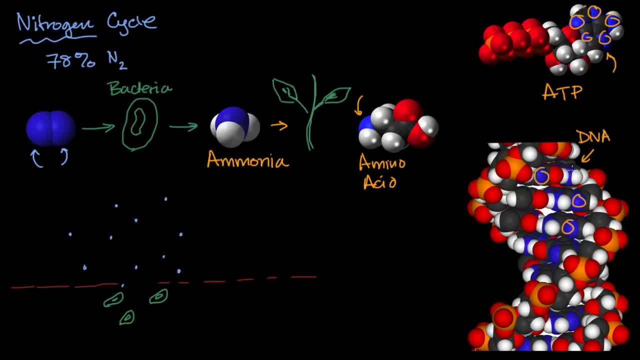 And you see the nitrogens throughout this macromolecule. So nitrogen is essential for life. but the step of fixing that nitrogen, that's done by bacteria, which can then produce the ammonia which is then usable by plants and then by eating the plants. 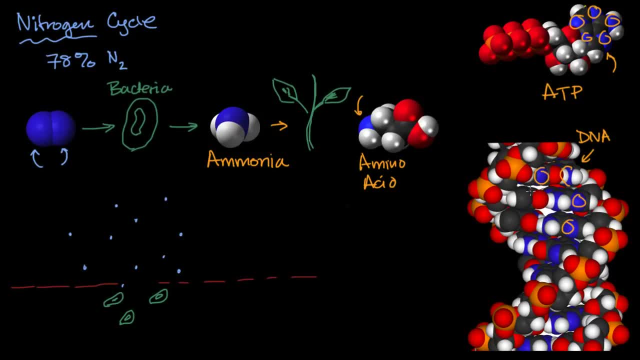 things like you and me can get that nitrogen into our systems. Now, it's not just a one-way system, It's not just a one-way street. We're just going from the nitrogen to the atmosphere and it gets fixed by prokaryotes. 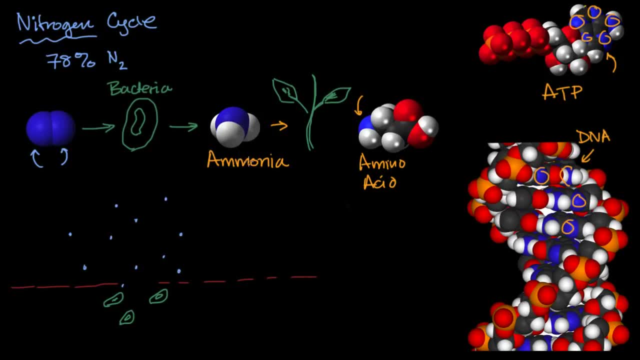 and then that gets used and that gets turned into ammonia and gets used by higher organisms, because then eventually all of it would get depleted As an organism dies as an organism dies. so let's say this is a dead organism. It could be a bacteria, but I'll do a higher organism. 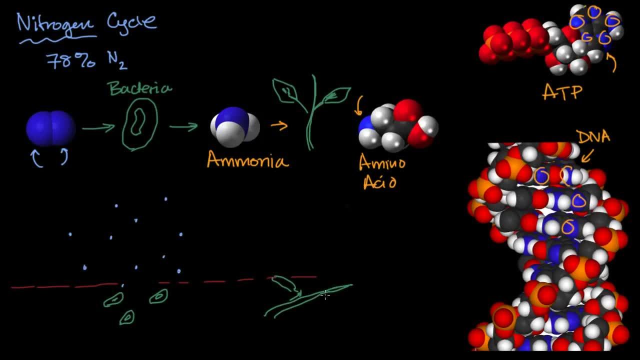 a multicellular one, This is a dead plant. here I don't want to draw dead animals, It's more morbid. So let's say: this is a dead plant, This is a dead plant there, and when it gets decomposed. 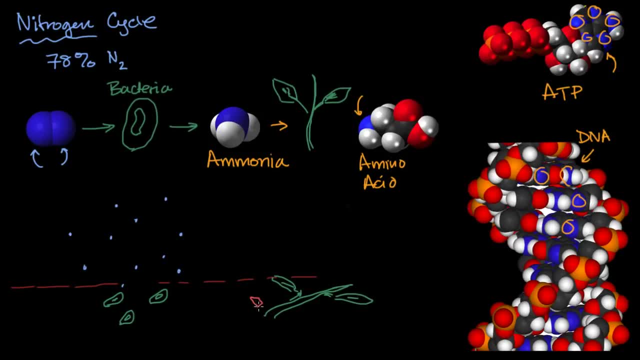 and there are many different types of bacteria, even though I might draw them looking kind of the same. Let's say this is another bacteria in orange. As these bacteria digest these plants they're able to. they could take some of the nitrogen and break them down into nitrites and nitrates. 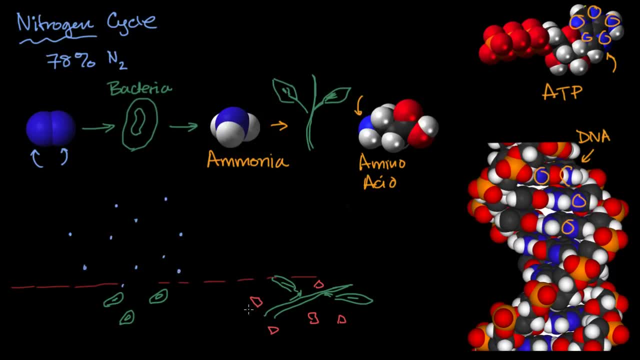 These are molecules involving a nitrogen bonded to two or three oxygens and they could take them back to ammonia. So we could go back, So we could have bacteria that take us back to ammonia, or eventually, by converting the nitrogen into nitrites and nitrates. 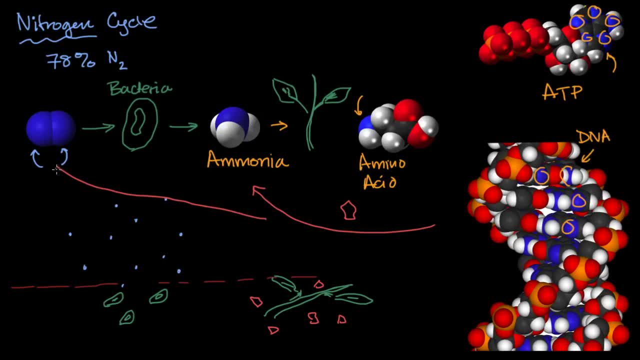 we could go back. we could go back to that molecular nitrogen, that N2, that then gets released back into the atmosphere. So or it could get, even, you know, it could get stored in other ways as well. But in general, as you see here this pattern, 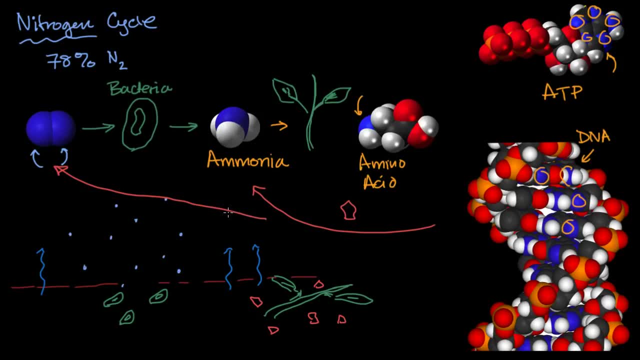 that we have these elements that are essential for life. they don't just disappear or form out of nowhere. They're constantly being recycled in our biosphere, And nitrogen doesn't get as much attention as carbon or oxygen, but it is essential for life. 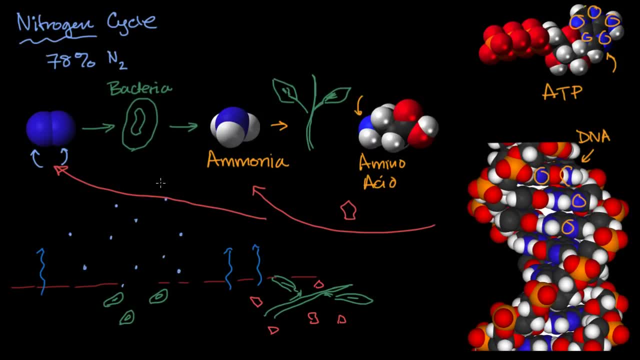 In fact, when you look at especially plants and growing plants and you think about fertilizer, fertilizer is something that if you think, if you add it to a plant it's going to grow more, So without it it kind of limits how fast a plant can grow. 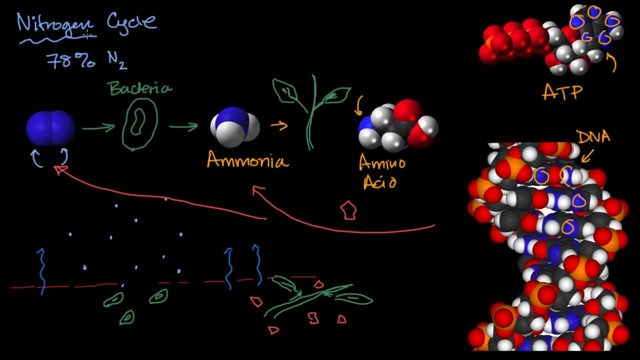 A lot of fertilizer is gonna have nitrogen and in another video we're gonna talk about phosphorus And that phosphorus and nitrogen and their availability in the soil is often a rate-limiting factor for plants, And you know that because if you add more nitrogen, 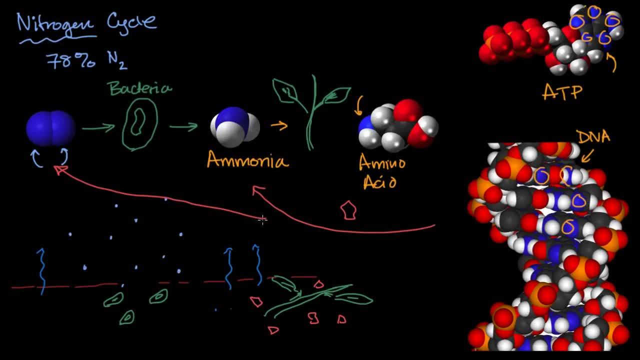 or that phosphorus. add more ammonia to that soil you're going to. the plants are going to grow faster.